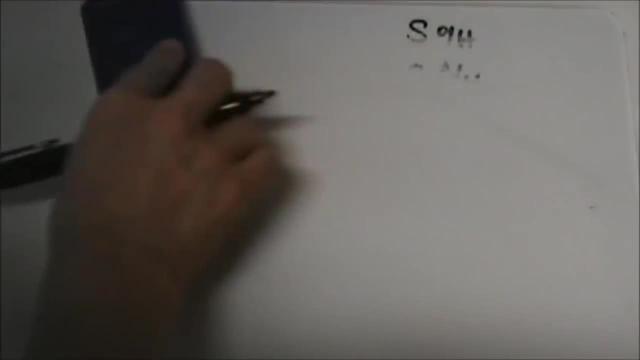 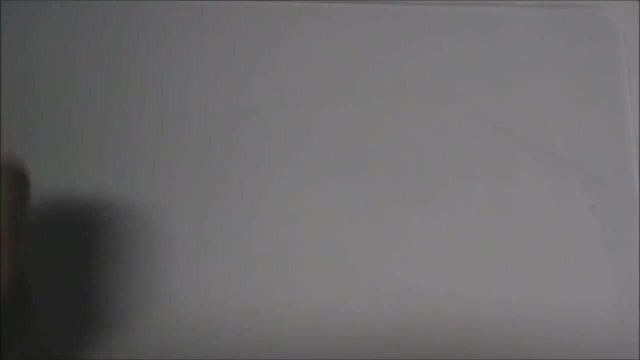 Not solving them yet, just setting them up. So I am going to jot this down for later. We have: the tangent of 52 is equal to 12 over x. So now let's look at the practice problem here. So here is our right triangle. we have a 48 degree angle here, so that is our reference. 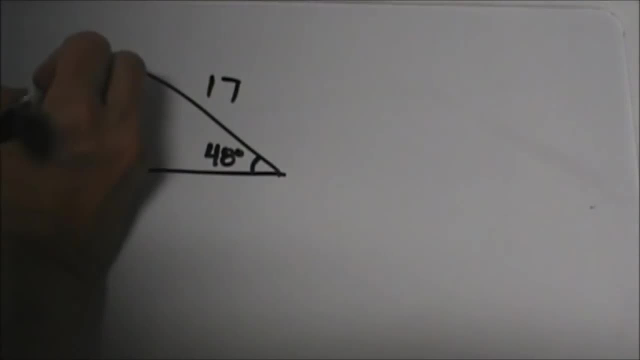 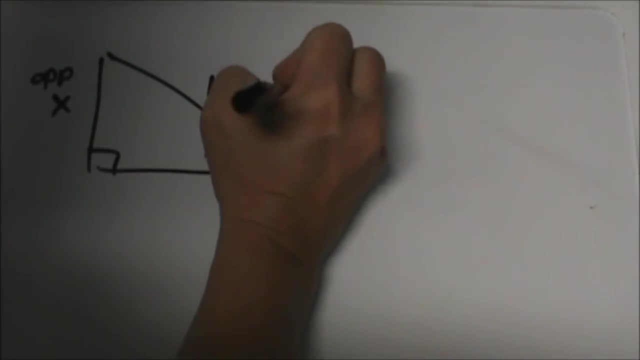 angle We have 17 on this side and x on this side. So from this reference angle, which two sides are we dealing with These two. So from here, this side, x is the opposite and the side that is marked 17 is the hypotenuse. 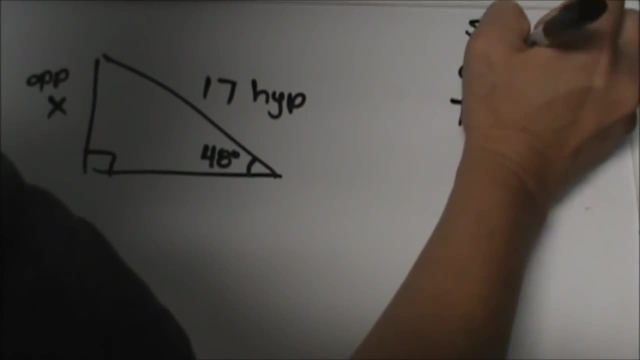 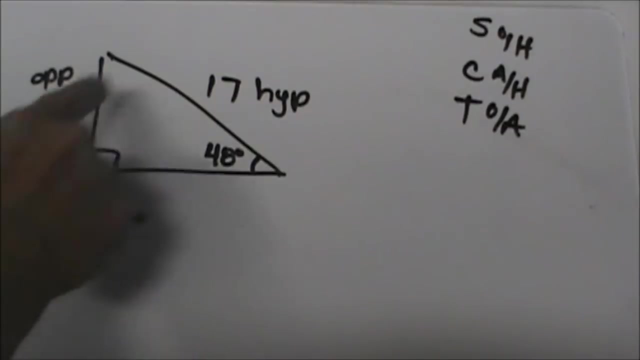 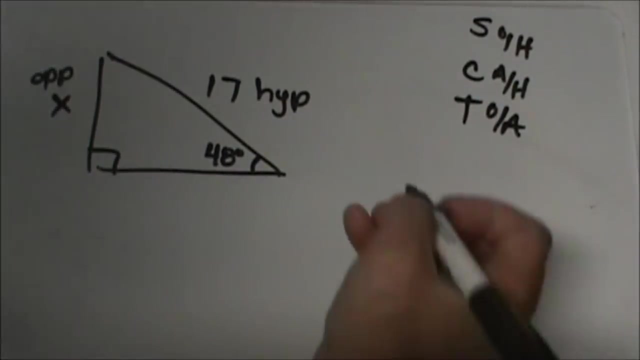 So we add sine and cosine, and I will try not to erase them this time. And which trig function uses the opposite and the hypotenuse? Well, that is the sine function, Because sine is opposite and hypotenuse. So I am going to set up the sine. of what angle? 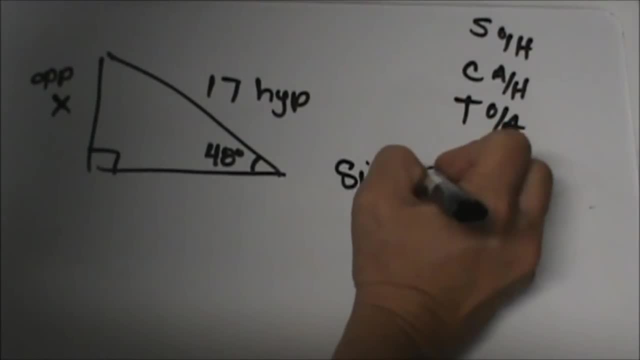 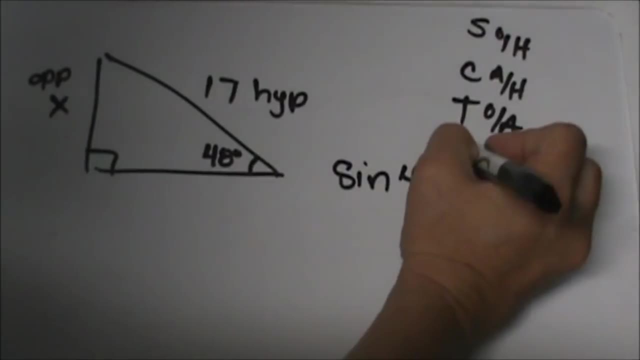 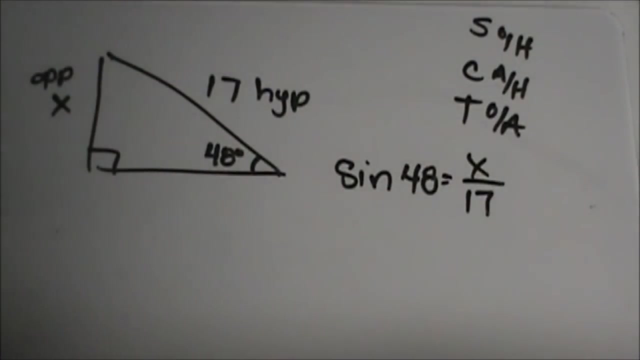 What is my reference angle? It is 48 degrees And that is equal to the opposite. So my opposite is my unknown. So it is on top and my hypotenuse is on the bottom and the hypotenuse is 17.. So the first problem is going to be: the sine of 48 is equal to x over 17.. 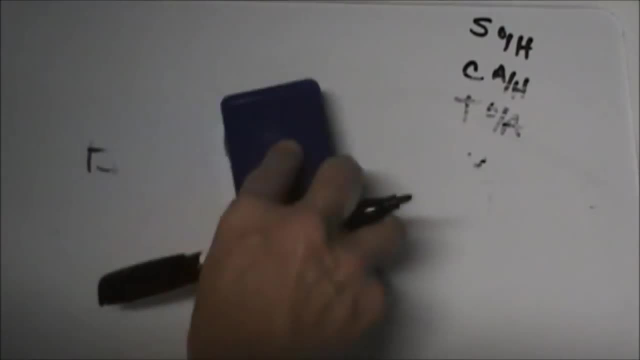 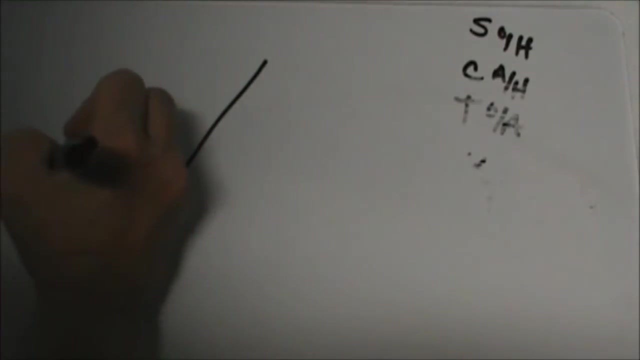 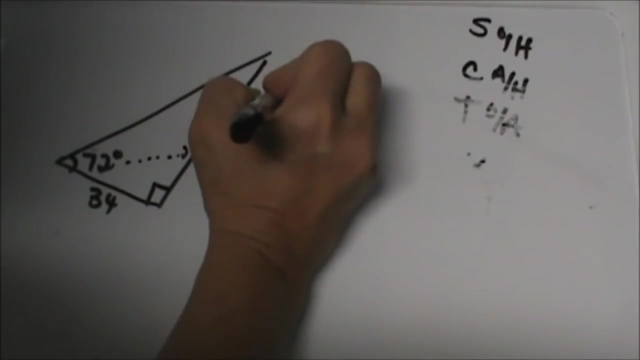 Let�s try the second practice problem. on your second page We have a 72 degree reference angle and we have 34 over here and x over here. So from the 72 degree angle, x is our opposite. This is our hypotenuse. 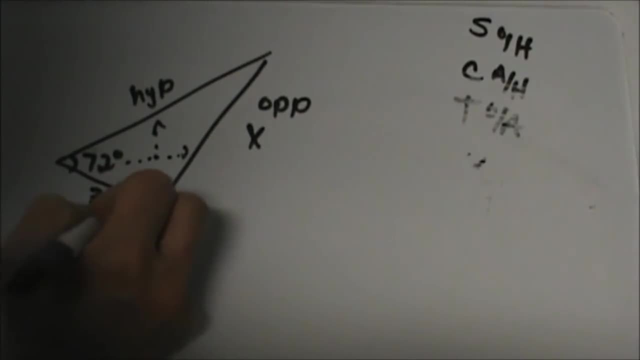 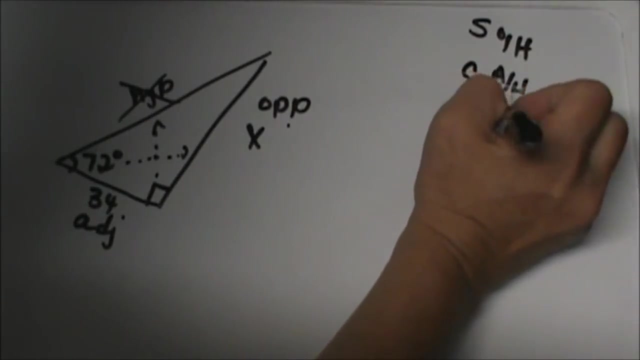 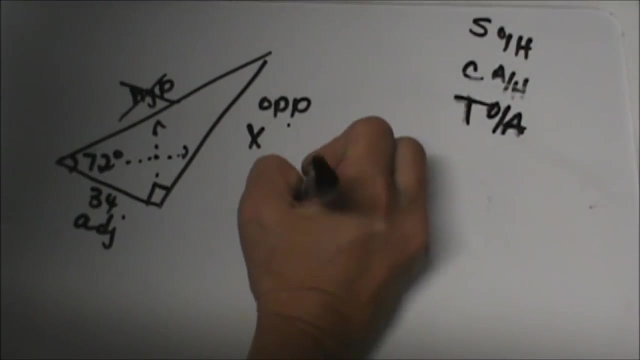 And this is our adjacent, so we are not using hypotenuse. So which one uses opposite and adjacent? Opposite adjacent is tangent. So let�s see if you can do this. We are going to set up the tangent. of what angle? Tangent of 72 is equal to the ratio of which two sides 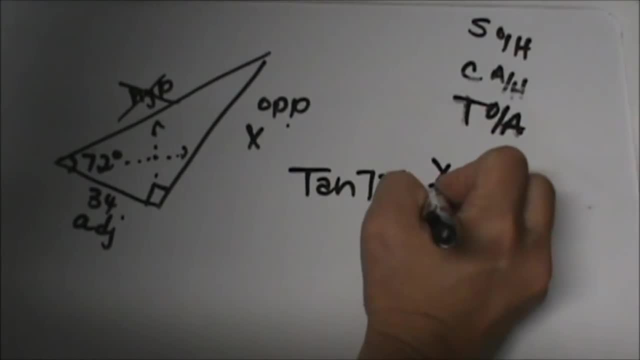 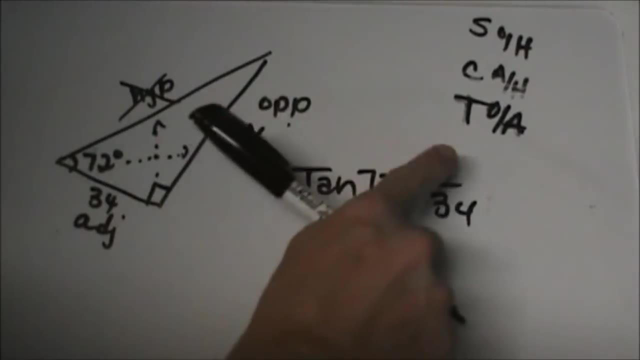 Opposite over adjacent. So I am going to have x over 72. So I am going to have x over 72. So I am going to have x over 72. So this one sets up as the tangent of 72 is equal to x over 34.. 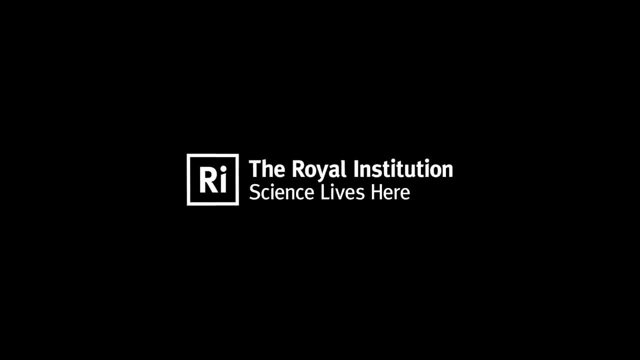 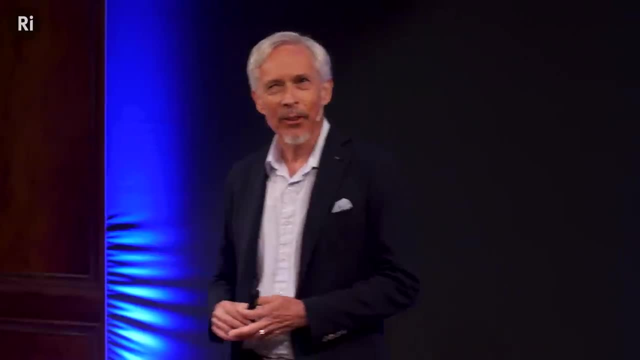 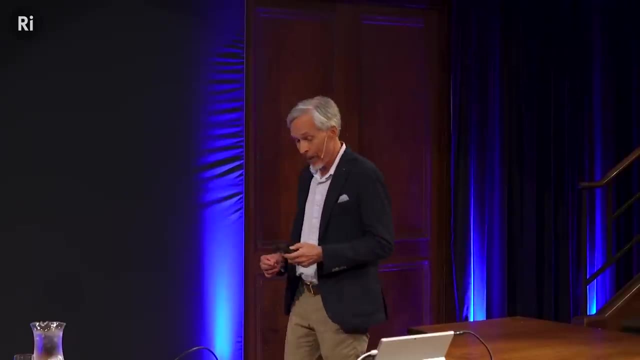 Thanks, Thanks, Peter. I'm delighted to be here. I first lectured here, I think six or seven years ago, about the future of space and did black holes during COVID. That was an online And today I'm going to talk about, I think, one of the most exciting subjects. I'll be a little presumptuous. 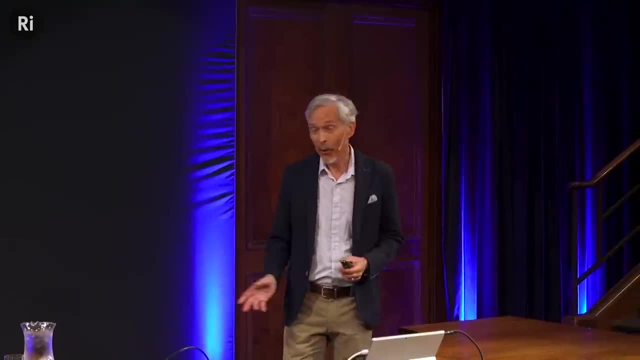 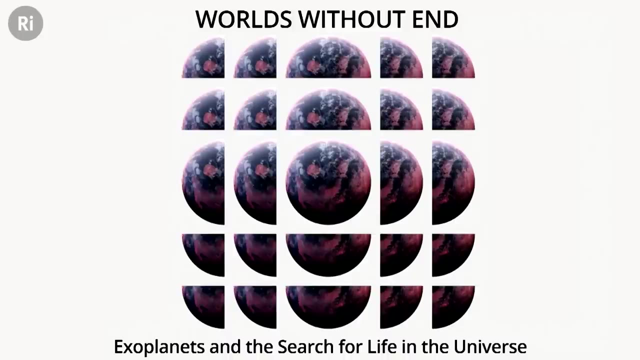 not just in astronomy but in all of science, which is the search for exoplanets, And I'm going to frame it more broadly as the search for life in the universe and give you a sort of status report on that. So I work at the University of Arizona And right away the whole search for 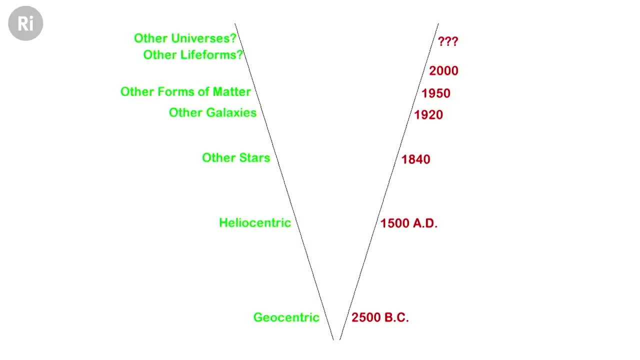 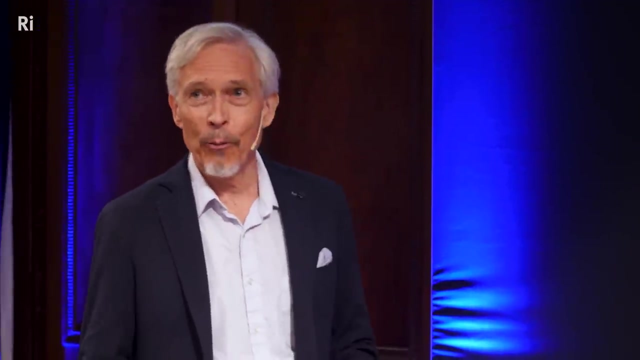 life in the universe, if successful, is essentially continuing the Copernican revolution. So the history of astronomy since Copernicus is to displace us in centrality in the universe. We're not special. We're not special in the solar system. Our galaxy is not special in a universe. 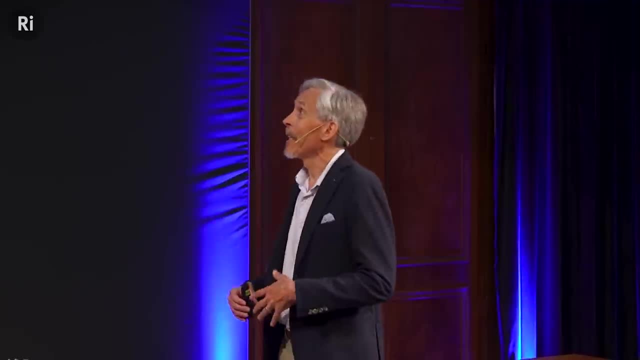 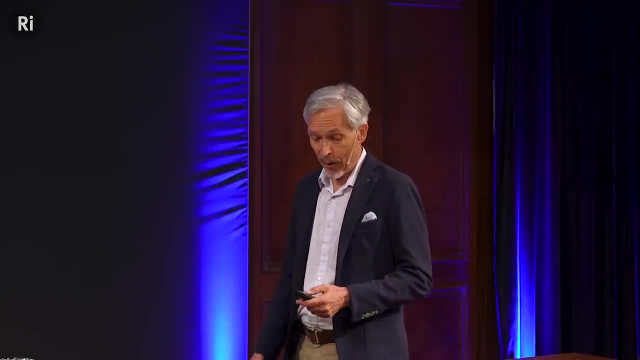 with hundreds of billions of galaxies, And so it would be consistent with this evolution of the Copernican principle if life were not unique to this planet. And so it's a compelling question to answer in science, I put, since I'm a cosmologist, I also put in there the fact 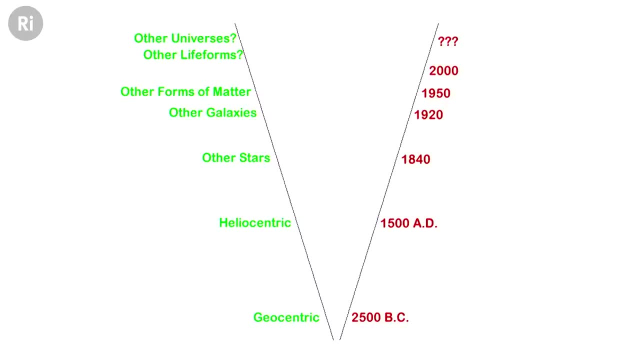 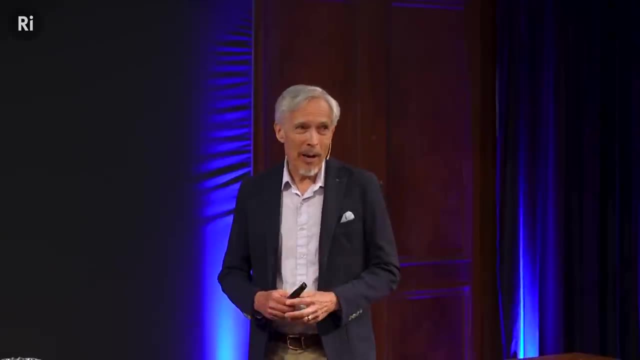 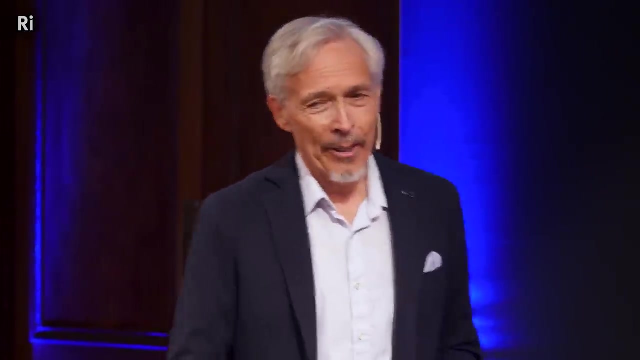 that there might be parallel universes, the multiverse, That's another talk. But astrobiology is really an exciting subject, but it has no subject matter. This is the only place in the universe we know with life, this planet. So why are astronomers fairly confident that we're? 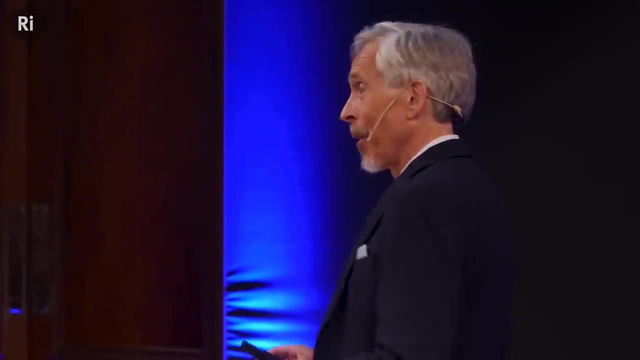 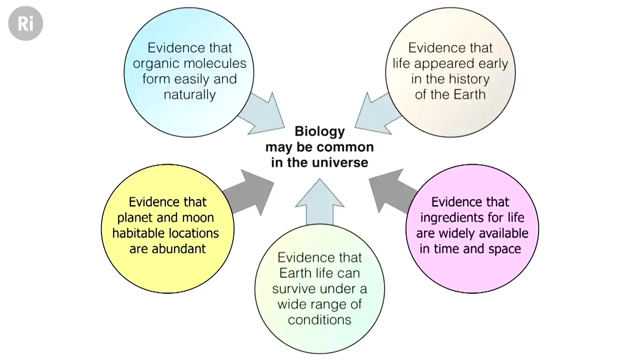 going to detect it elsewhere soon, Not just within all of our lifetimes, perhaps within the next few years. It's a series of indirect arguments, The fact that the ingredients for life are widely available. Carbon is made by stars everywhere in the universe. Water is one of the.